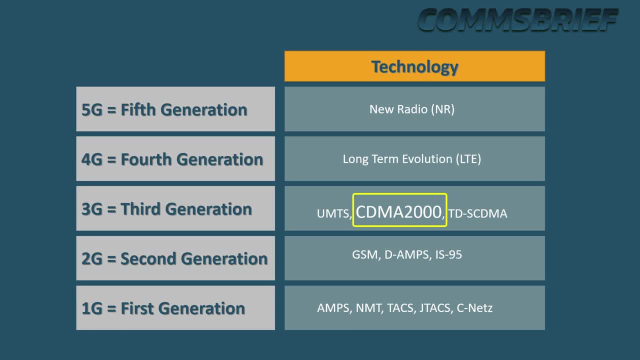 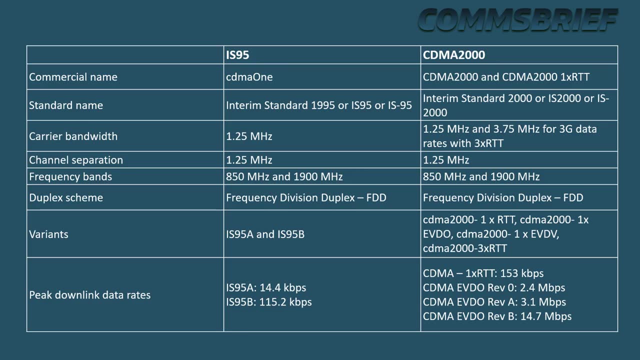 of mobile networks. As you can see, CDMA 2000 is one of the key 3G technologies, just like UMTS. Let's now have a look at this table, which may look a bit busy when you first look at it, but let's go through these rows bit by bit. 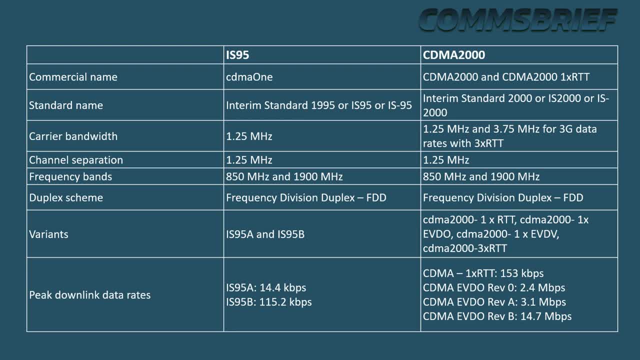 to understand it clearly. So one of the best ways to learn about a new technology is when you compare that with an earlier technology, and that's what we will do here. We'll compare CDMA 2000 with IS95.. So if you look at the second row, the technology standard that defines CDMA 2000. 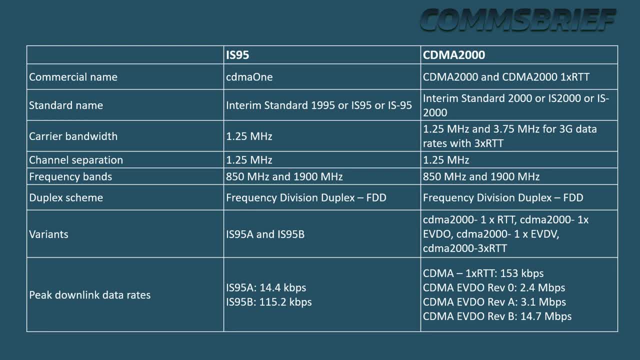 is IS200. And so, with this information, we can see that it is based on the IC put on the device, but instead of IS200, we can also see that it is based on the IC added to the device, the IC that we are currently using. 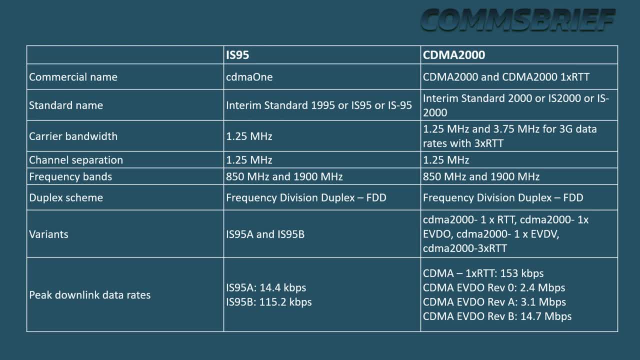 so this is called the IC. basically that is the CDMA 2000, Interim standard 2000.. Just like CDMA 1 is IS95, and that is because IS 2000 was introduced in the year 2000,. 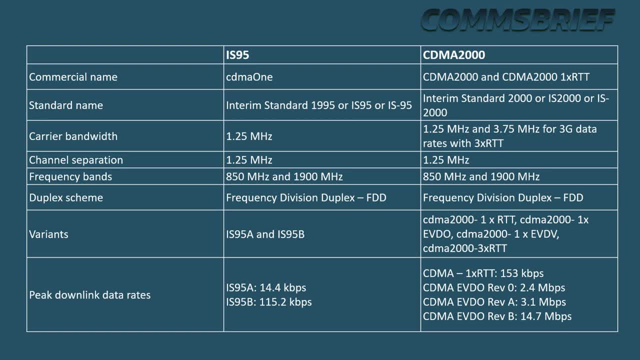 whereas IS95, as the name suggests, was introduced in 1995.. CDMA 2000 is backwards compatible with this predecessor, IS95, making the upgrade from IS95 to CDMA 2000 easy and seamless. The bandwidth of these devices is 4.6 megabits. 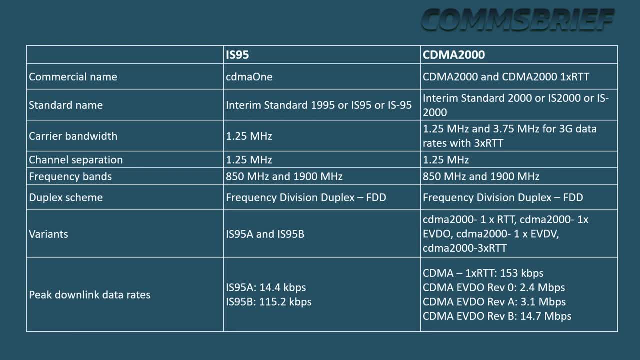 In contrast, CDMA 2000 is less than 2 years old, while this is the same as CDMA 2000,, homologous in terms of performance, performance, performance and performance. The bandwidth of each channel or carrier is important, because that is what gives you higher data rates. 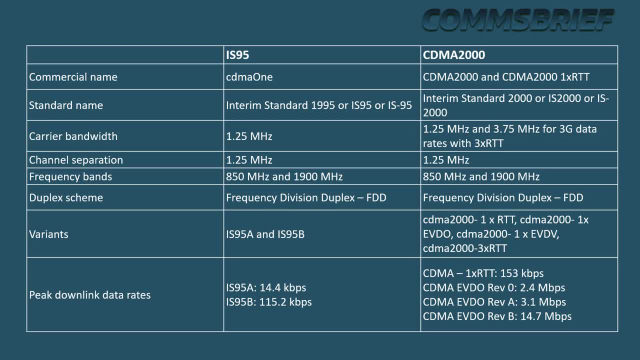 In IS95 or CDMA1, the bandwidth was 1.25 MHz, but CDMA2000 is able to aggregate up to three 1.25 MHz channels to get a total bandwidth of 3.75 MHz. Just for comparison, in UMTS, which is the GSM version of 3G, you generally get a bandwidth of 5 MHz. 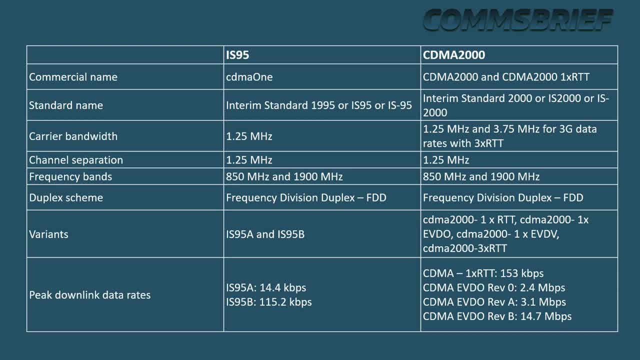 So UMTS has flexible bandwidth as well, but 5 MHz is the general or most common bandwidth that is used. CDMA2000 networks can operate in both 850 MHz and 1900 MHz frequency bands, just like the earlier IS95 networks, with separate frequency bands for uplink and downlink. 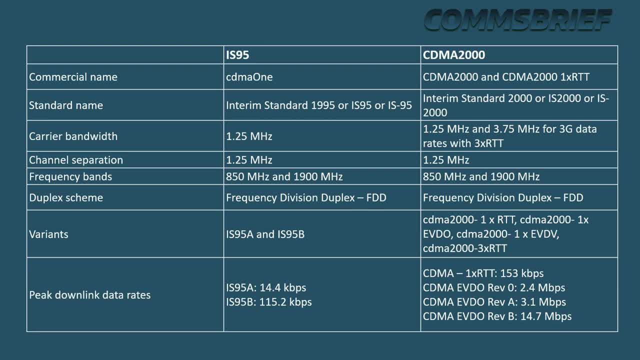 The uplink in CDMA is called reverse link and the downlink is called the forward link. CDMA2000 has seen several enhancements, including CDMA2000 1x- EVDO- evolution data optimized. CDMA2000 1x- EVDV- evolution data and voice. 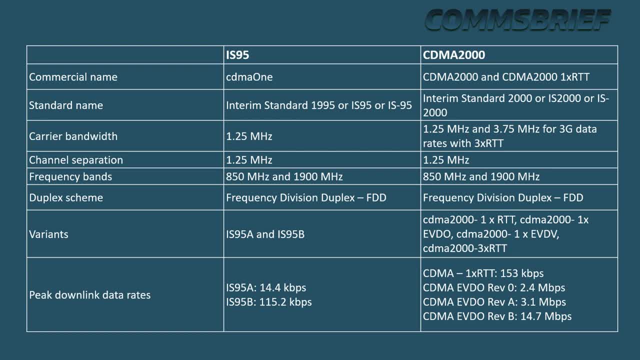 and CDMA2000 3x RTT, which is 3x radio transmission technology, which means three carriers are used: 1x RTT. 1x RTT can support peak data rates of 153 kbps in the downlink and the uplink. 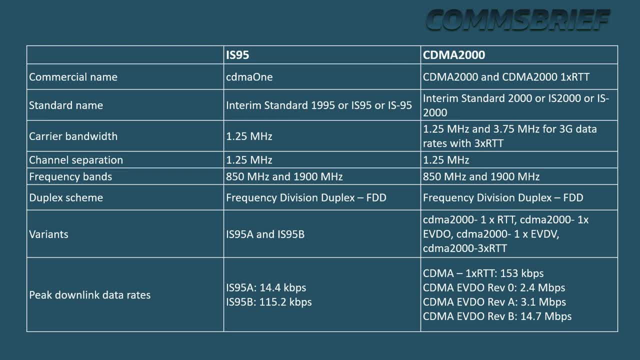 So 1x RTT means one carrier of 1.25 MHz is used. And finally, with the EVDO revision B enhancement, CDMA2000 can support maximum data rates of up to 14.7 Mbps. Before we finish, let me take you through one more concept. 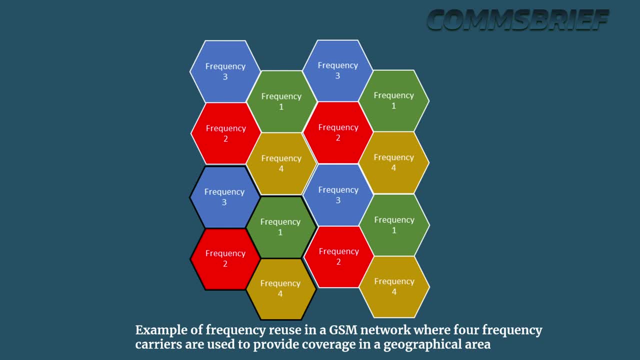 The networks. Before CDMA, mobile networks were using a combination of FDMA and TDMA4 radio transmission, So that is what GSM and D-AMPS networks used. The challenge with that is the potential interference caused by the same or adjacent frequencies. 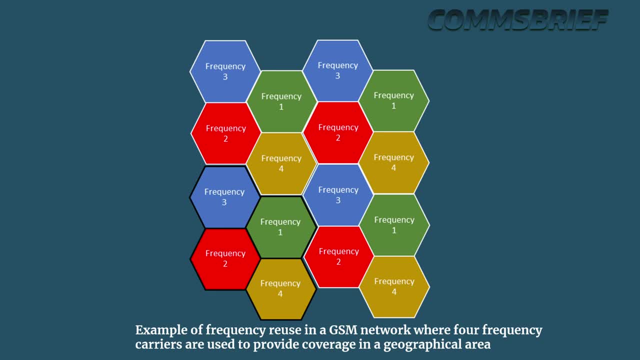 These interferences are called co-channel and adjacent channel interference. As a result, when RF engineers are planning the cells, they make sure they reuse the frequency channels carefully to ensure that when they assign a frequency channel to a cell, they avoid using the same or adjacent channels in the neighbouring cells. 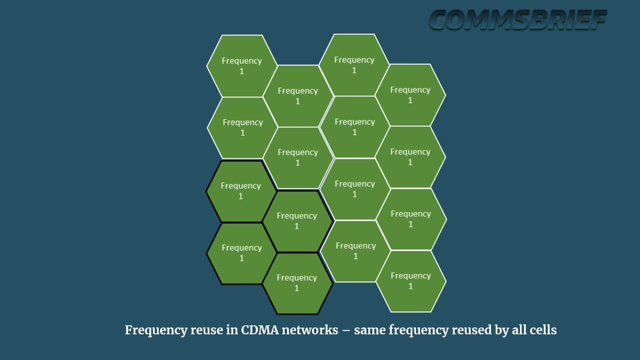 Now, CDMA networks do not have the frequency reuse limitation and they use the same frequency carrier or channel in all cells, Unlike TDMA, FDMA-based networks like GSM and D-AMPS, where a handover requires a mobile network. 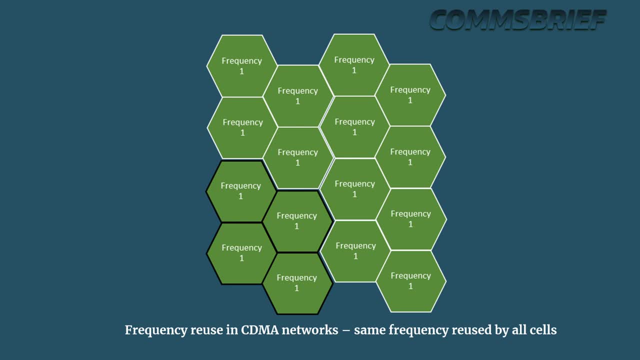 it requires a mobile phone to disconnect from one cell before connecting to the new cell. CDMA networks use a concept of soft handover or handoff. Since CDMA networks use the same frequency across all cells, a mobile phone can communicate with multiple cells simultaneously.